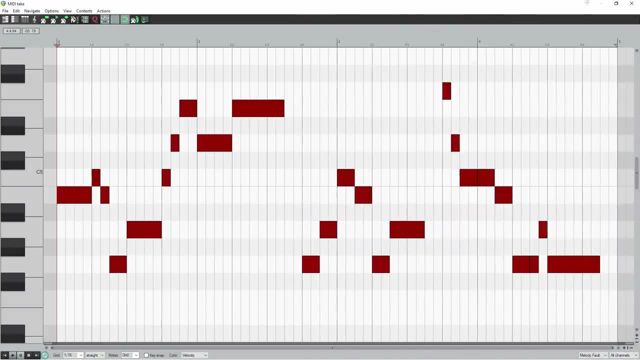 So what's the fault in this melody? Well, it sounds completely lifeless, right? It's totally lacking in vital energy. What's causing that Rhythm? Or rather a lack thereof? Unfortunately for rhythm, it's usually the overlooked element in a melody. Indeed, 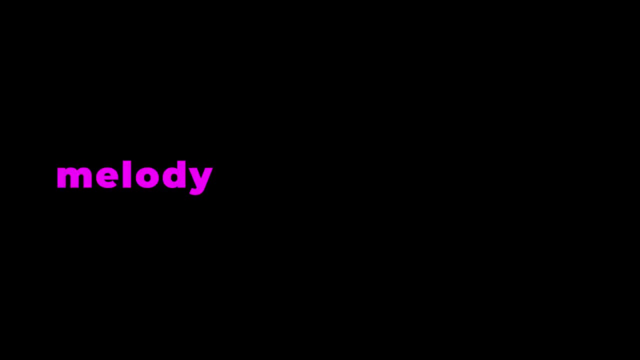 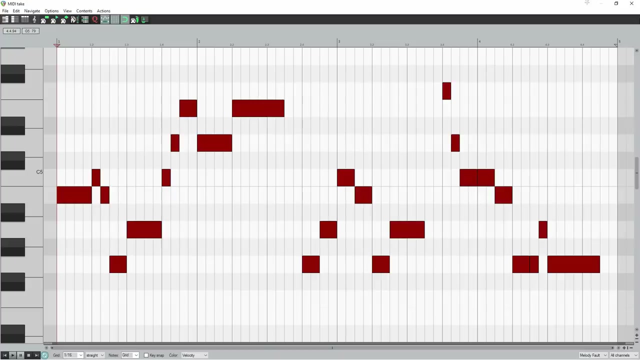 songwriters and producers often seem to forget that melody actually contains two elements: pitch and rhythm. To hear this in action, just listen to the New Music Friday playlist on Spotify every week. It's clear that the rhythms of most melodies are an afterthought at best. 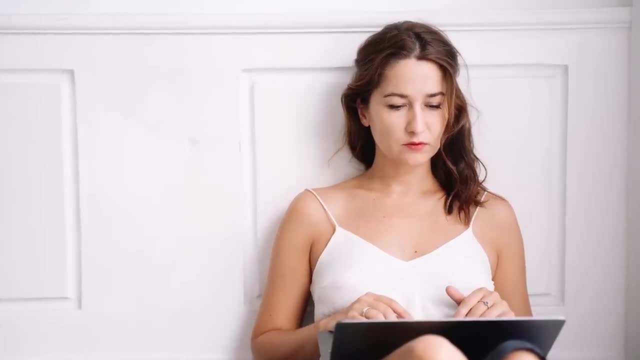 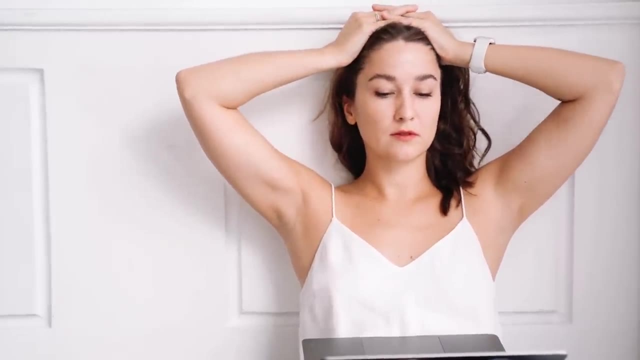 Mhm. I've worked with countless songwriters and producers who've ended up at the horribly frustrating point of wanting to delete a melody because they just can't get it sounding. right Up until that point, though, they'd spent all their time trying to. 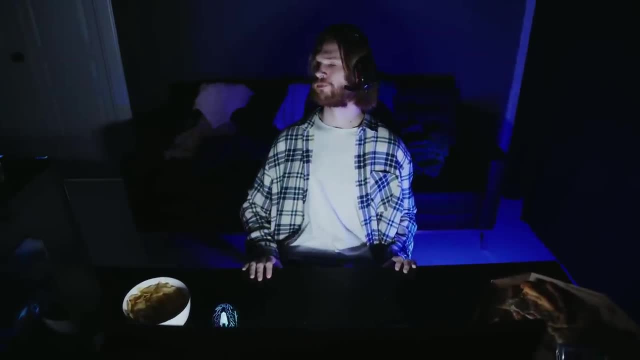 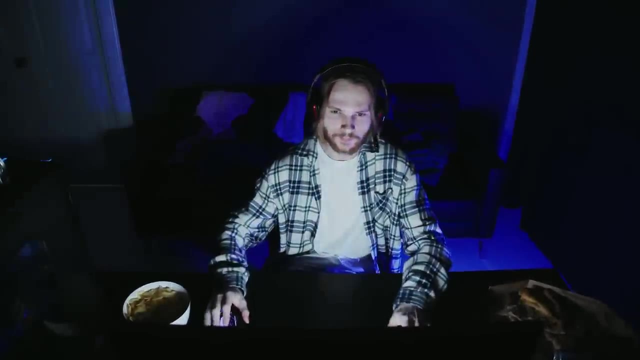 fix the pitches, but they'd not once considered that maybe it's the rhythm that needs fixing. So, after bringing their attention to the forgotten element of rhythm, a few small tweaks later and they've fallen in love with the exact same melody they were about. 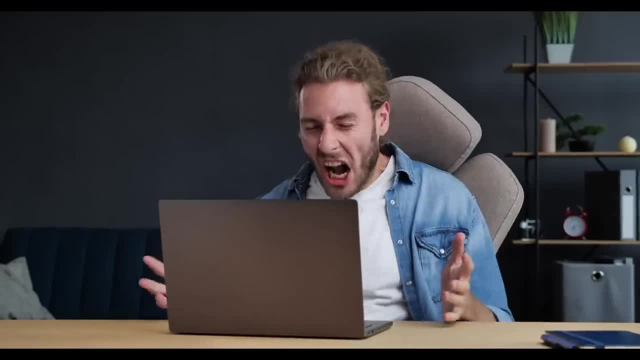 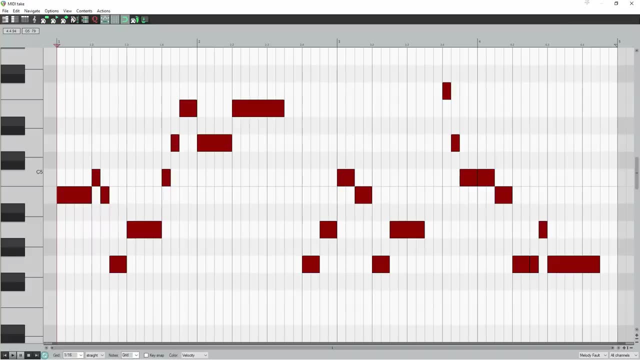 to delete. So next time you're frustrated and tempted to delete a melody, try experimenting with its rhythm instead and see if you can save it. Now you're back. You're probably wondering what exactly makes a good rhythm. Well, first, it's important to remember: 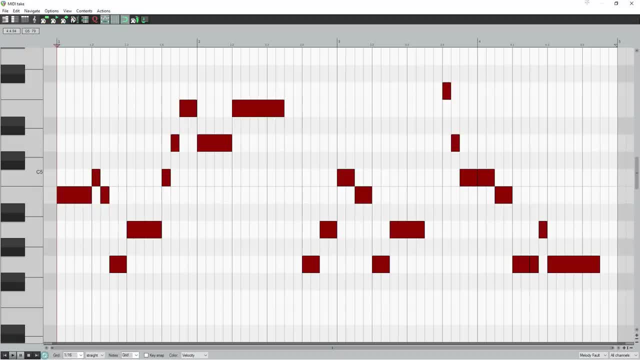 that a rhythm is a pattern in time And, just like with all other patterns, our human brains get bored if there's too much repetition and they get overwhelmed if there's too much variety. Therefore, good rhythms, like all good patterns, enjoy a pleasing yet interesting balance of repetition. 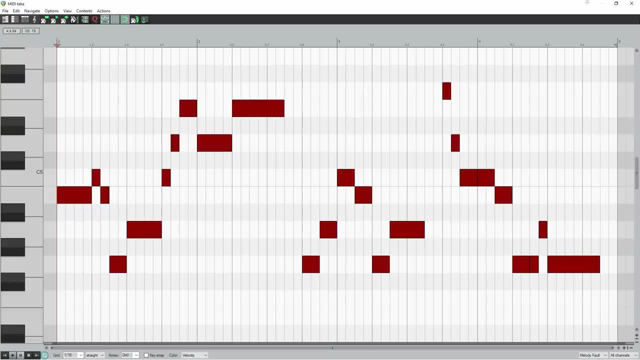 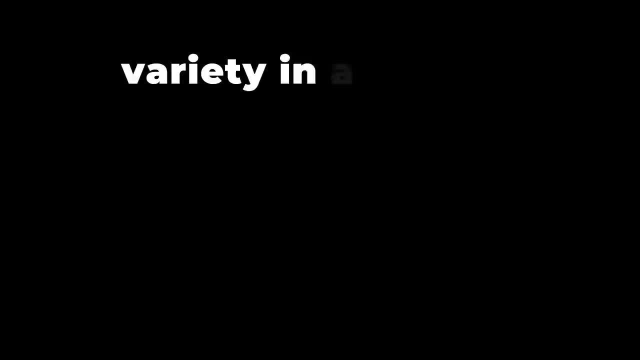 and variety. Mhm And most melodies these days do not have any problem with repetition. Okay, It's the lack of variety that causes their weakness, Mhm. Variety in a melody is created by using many different note values and, most importantly, syncopation. 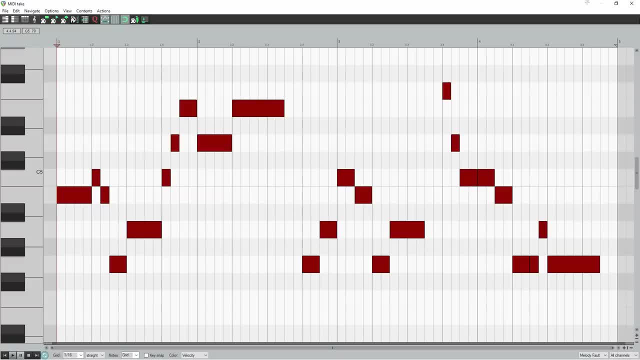 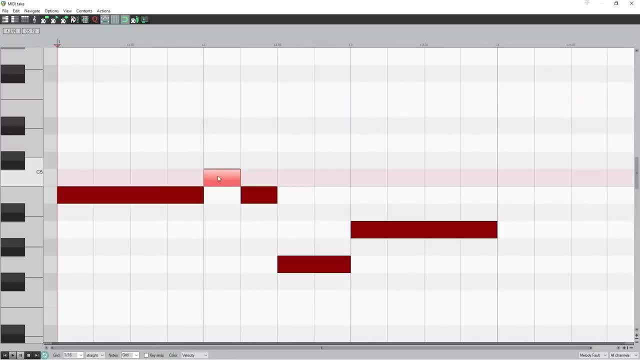 Syncopation is when you accent an offbeat and it puts a real spring in your melody's step, bringing it to life. For example, in the first three beats of our rhythm we move two on-beat notes to offbeats.